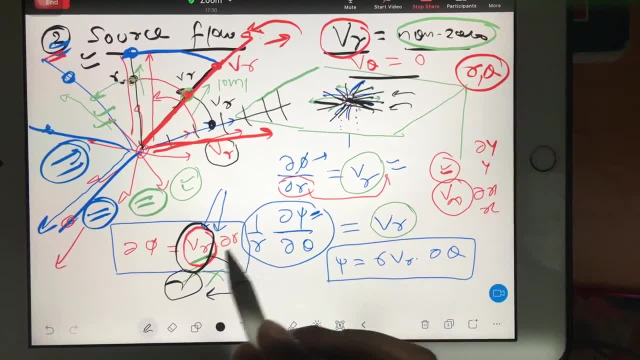 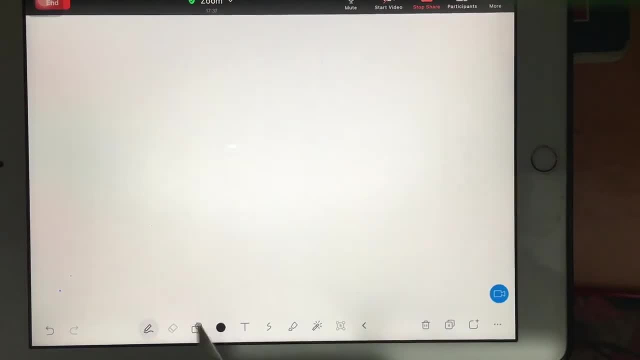 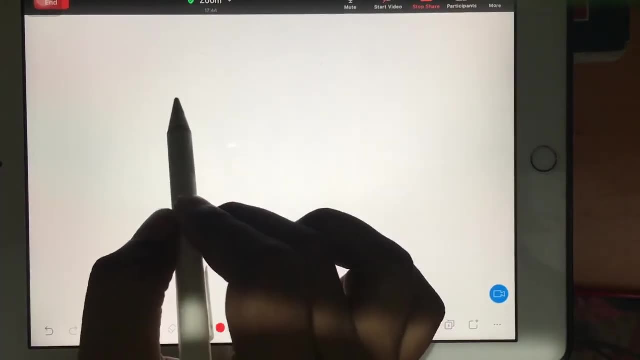 technique to convert our Vr in terms of r. So let's talk about that. So let's talk about that. So we must have some technique to convert our Vr in terms of r. Then only we can integrate for the r and same here. So it means we have some duty remaining for source flow. Let's go ahead Now. what to do? See, guys, everyone, Actually, we don't study this for a plane. Whenever we study source flow, we don't study for a plane. What do we do? Yes, Ranjith, ask it out. 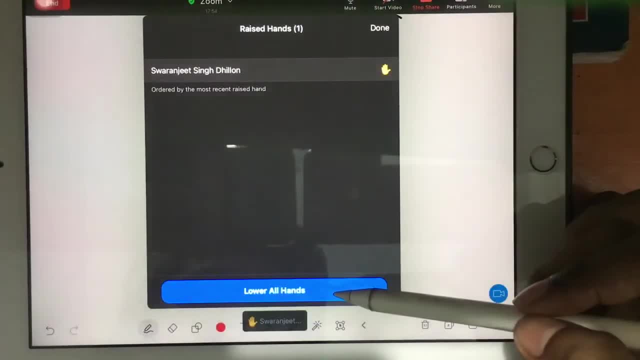 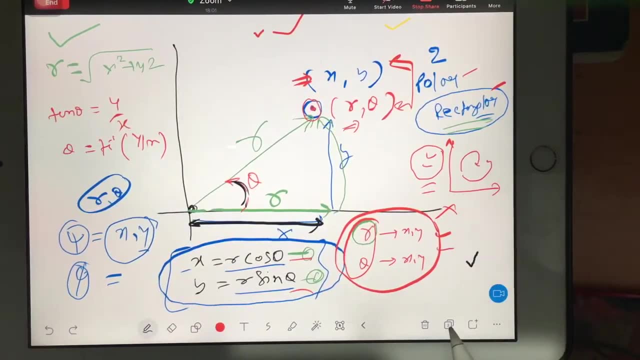 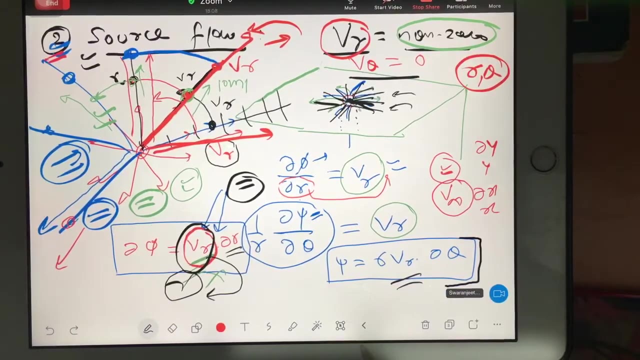 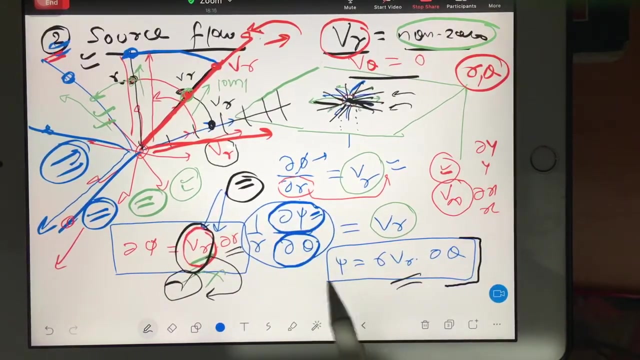 This one, This one, Which one? Yeah, yeah, okay, See here what I am saying, This formula: dou psi by dou theta. I am just rearranging in this way, I am simply rearranging. Now, after this rearrangement, I have to integrate. I have to integrate for d theta. But see, we cannot do this integration before knowing the nature of Vr. 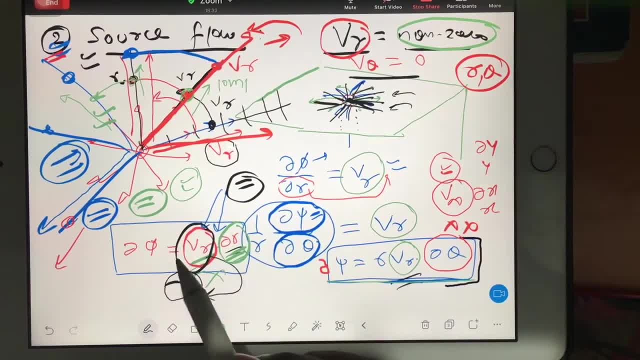 Here also. I am simply rearranging Here also. we cannot integrate dou R without knowing the nature of Vr. So during the theory when I was explaining, I explained that Vr is actually changing with radius. So if Vr is changing with the radius it means definitely we have a formula of Vr in terms of radius. 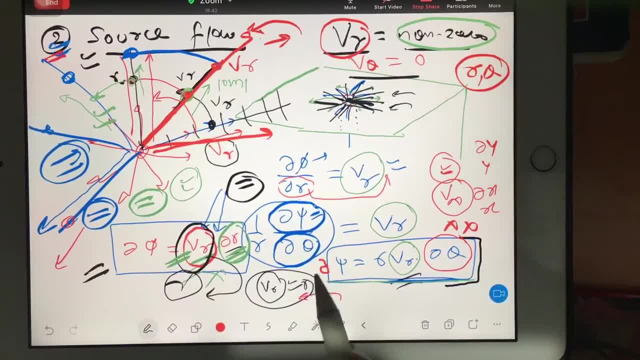 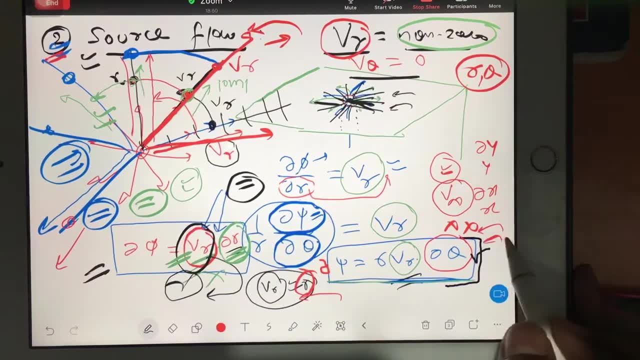 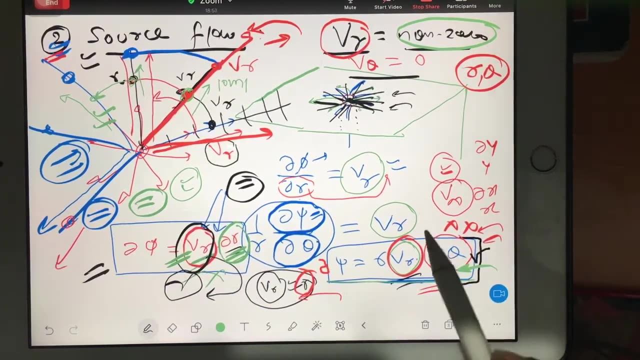 Oh, when I was explaining, I explained that we are is actually changing with radius. So if Vr is changing with the radius, it means definitely we have a formula of Vr in terms of radius. No, no, before integration itself, we have a trouble. We have not done integration yet. Before the integration itself we have trouble. and the trouble is Vr is not constant. 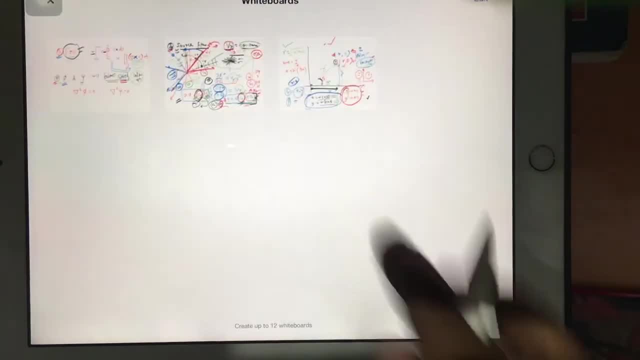 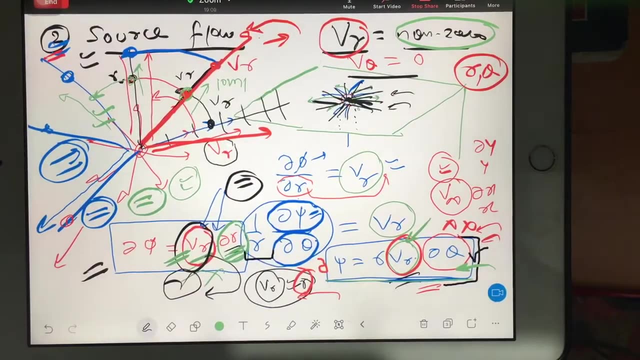 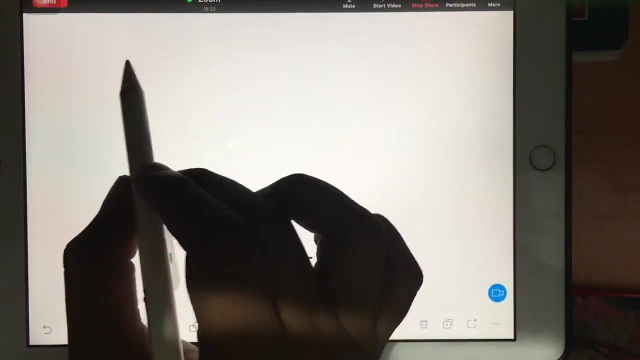 Try to understand my logic. That R we are going to discuss now. Oh no, no problem. That is that. see what I am saying. I will write again. I will write again. See what, what, what my approach is. My approach is: we have our dou psi by dou. theta 1 by R is: 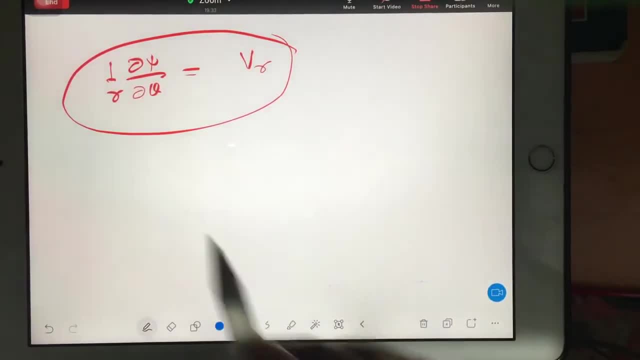 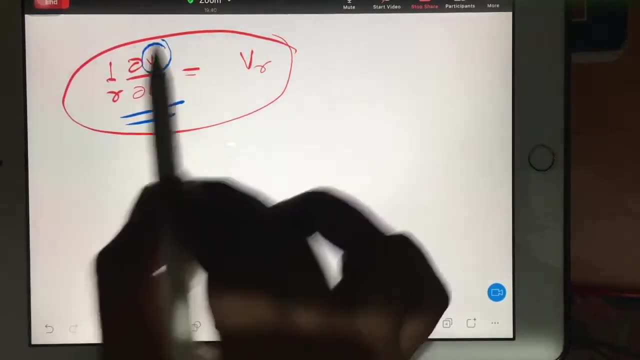 equal to V R as a formula. Now, in this formula, yeah, in this case. So I want to know, I want to know this: dou psi, sorry, the psi, So psi value is nothing but V R into this R into this dou theta. 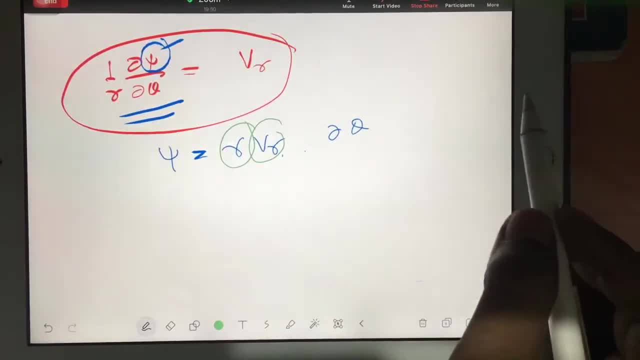 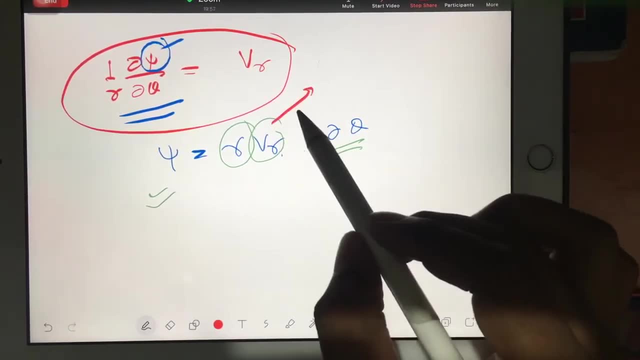 Now, if they both are constant, then you you can immediately integrate and you can develop the equation for psi. But there is the issue: during theory You got it right. So this V, yeah, yeah, very good. So this V R is actually. 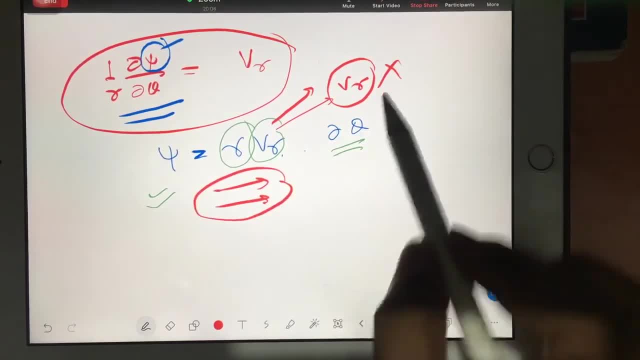 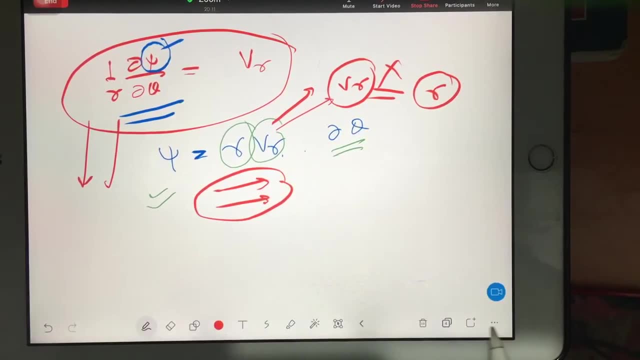 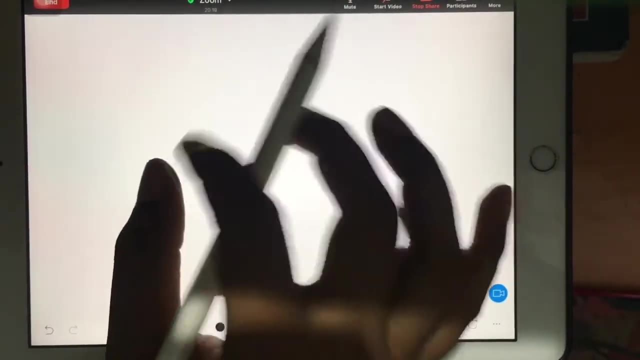 not constant. So now we are going to understand how to achieve V R equation in terms of R, Then only we will understanding this properly. So for that, so I am changing the page. See now. First thing: keep in mind whenever we are discussing source flow, we cannot study this. 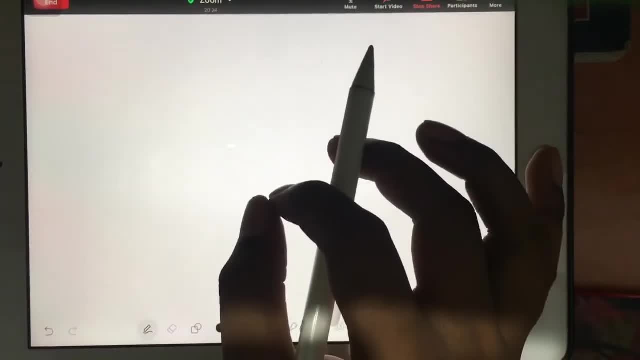 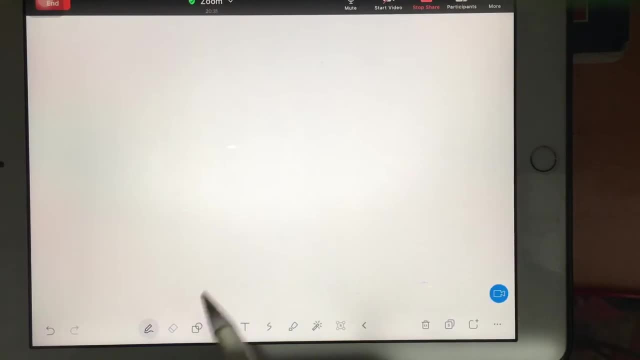 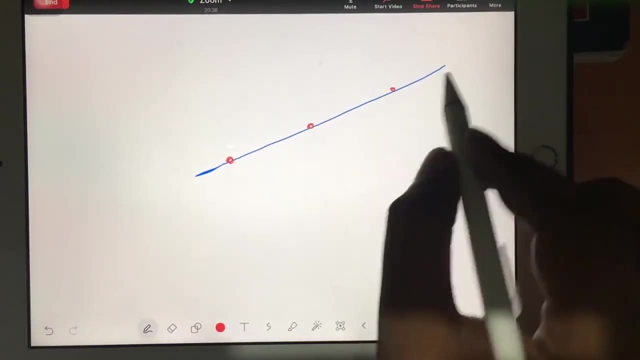 source flow in plane. So to to develop the source flow formula in terms of R, we have to assume a cylinder. So I'm drawing a cylinder. Now, what kind of cylinder I will draw, I will tell you I will. I will make an axis. on this axis I will put all the source sources here for the flow And you. 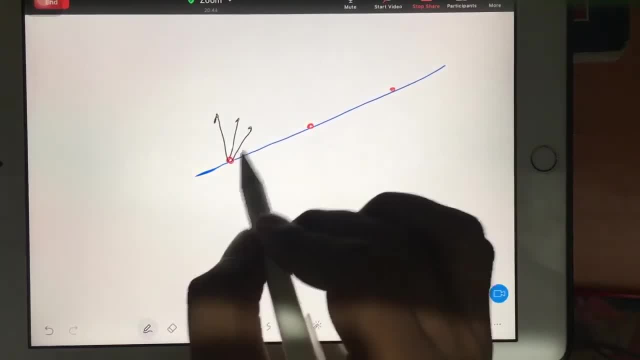 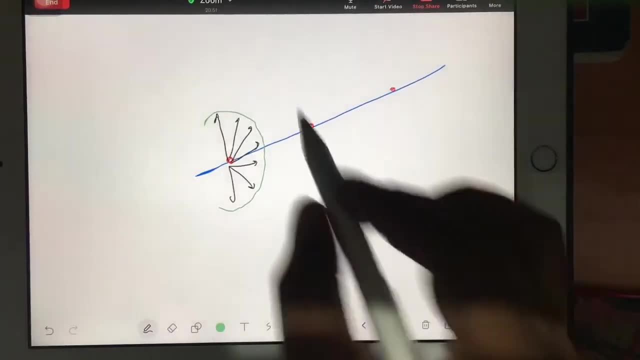 know the sources will be producing flow like this, like this. So what will I do? I will pack them in circle. Right In same way. I will pack them in circle, I will pack them in circle. So I have taken only. 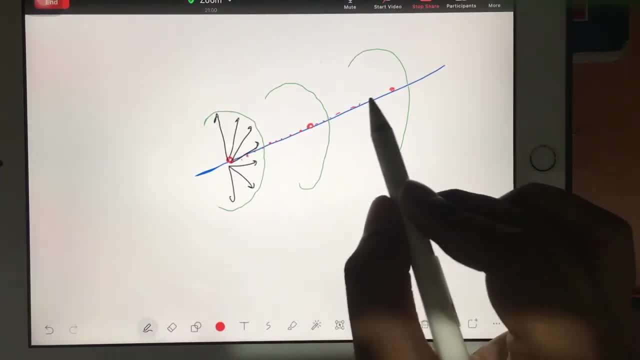 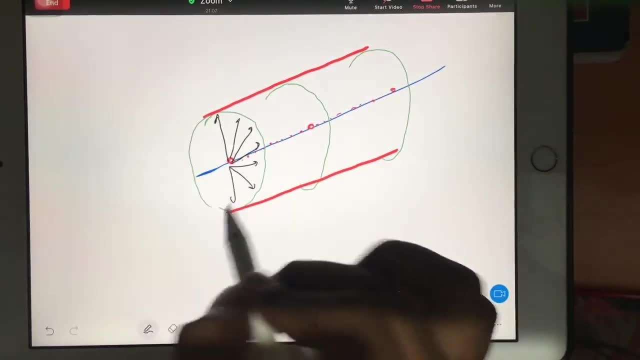 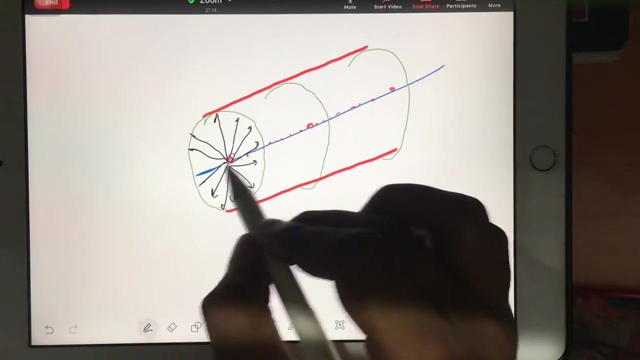 three points, but there there will be infinite sources in between infinite sources. It means what? It is actually a cylinder, right Now, you see it is actually a cylinder. Okay, Means this source flow, suppose I'm taking the example of water. So every source is producing. 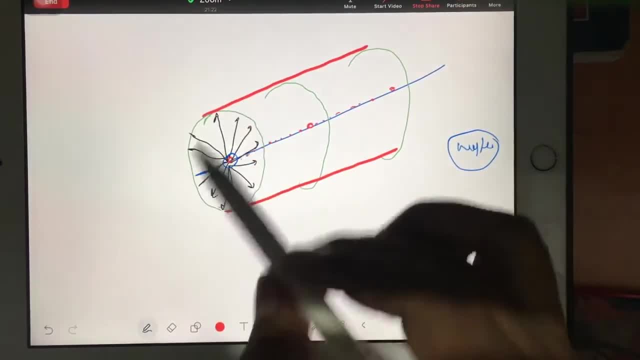 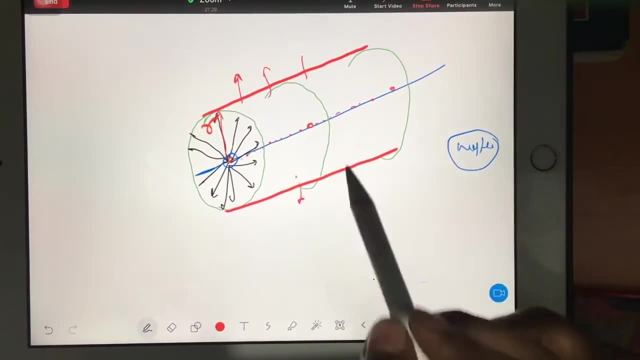 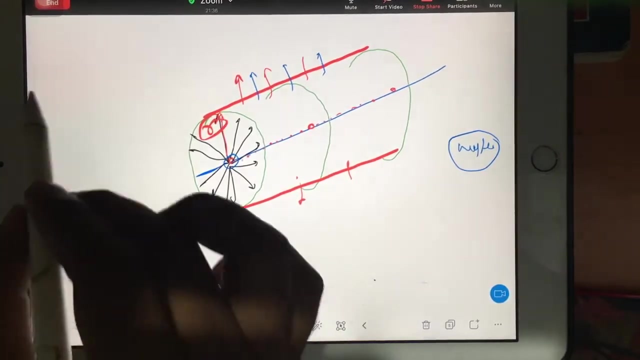 water means From the cylinder at radius R, for out of the cylinder your water is coming out. at radius R your water is coming out. It means that water will be having mass flow rate. You see how I'm developing the formula So that mass flow rate. you know how to write, always whenever we write. 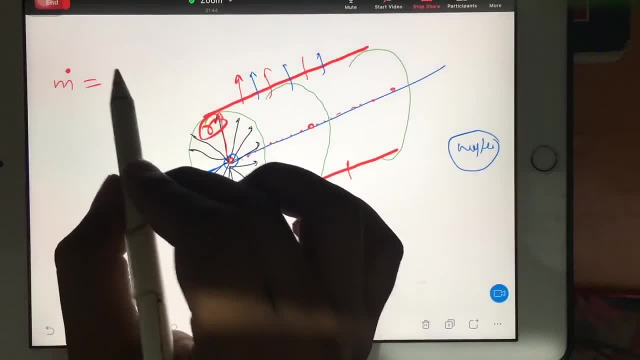 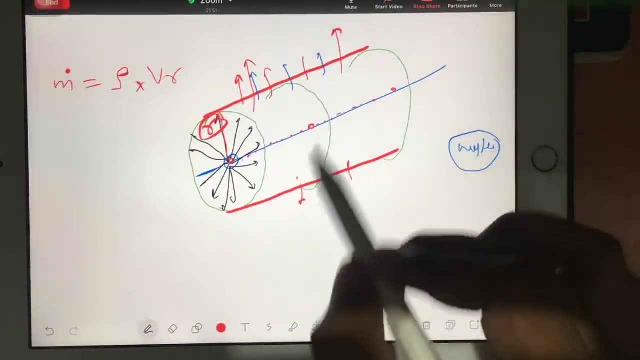 mass flow rate. we have formula row AV right. So row is going to be the density of the liquid And V is nothing but the radial speed of the water, because water is coming out in the direction with the speed of VR. You can see here VR, at this location, VR, now row, is over velocity. 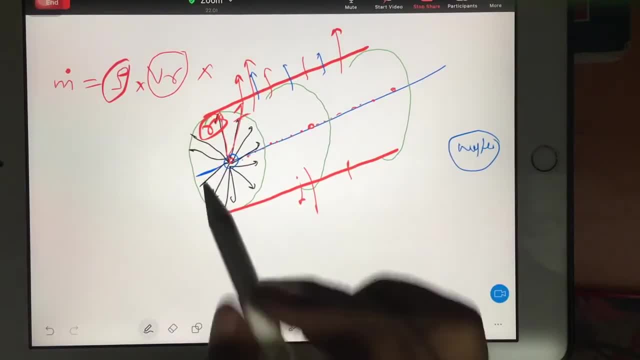 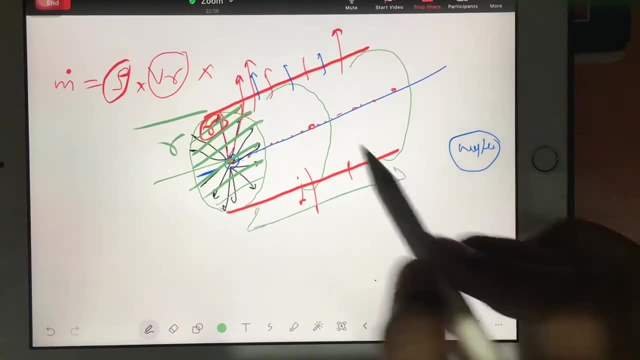 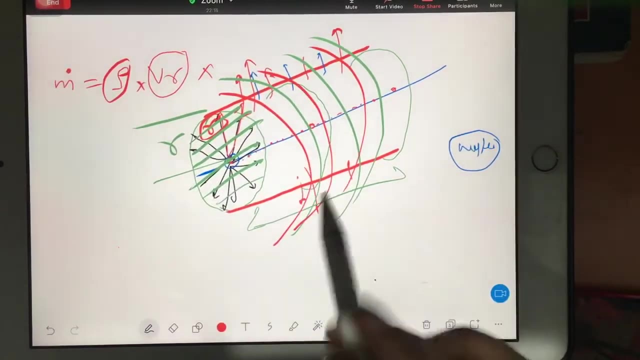 is over, but area is remaining. So we are targeting at radius R, correct? So this is nothing but a circle. you know what is the uh area of this curvature, of this curvature through which water is coming out? at a circle. can someone recall PI or L, PI or L. PI or L is totally wrong, PI or L is. 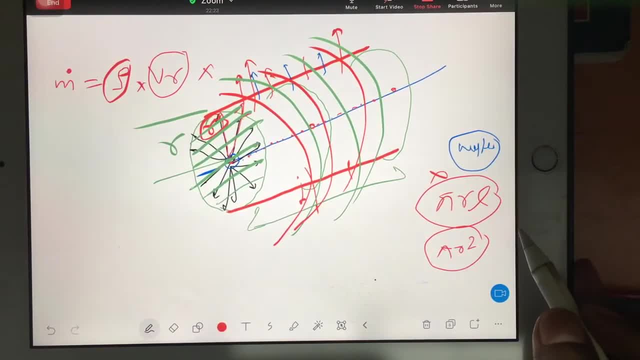 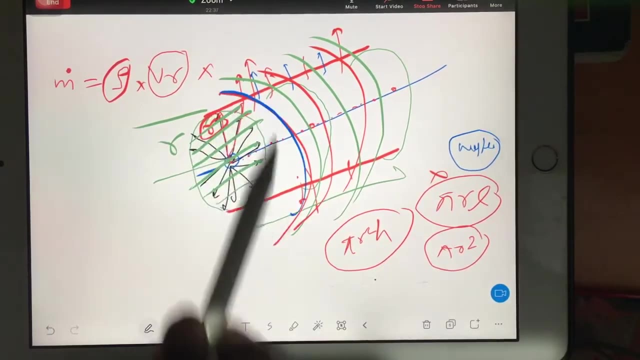 totally wrong, Push it, I suppose. Okay, Your cap, Your cap, Your cap. totally wrong, Totally wrong. Pi r square is totally wrong, Man, what you guys are doing. Seriously, I am asking: area of this curvature, Pi r square, is you check out the unit, man? 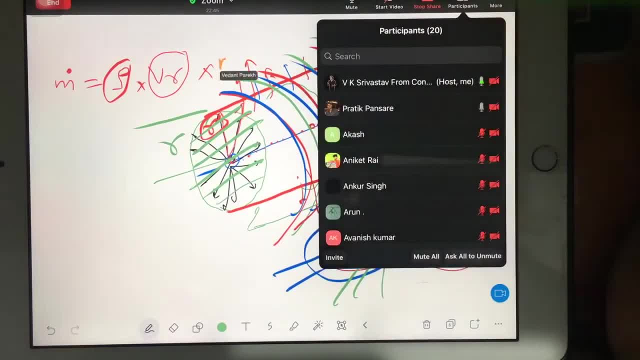 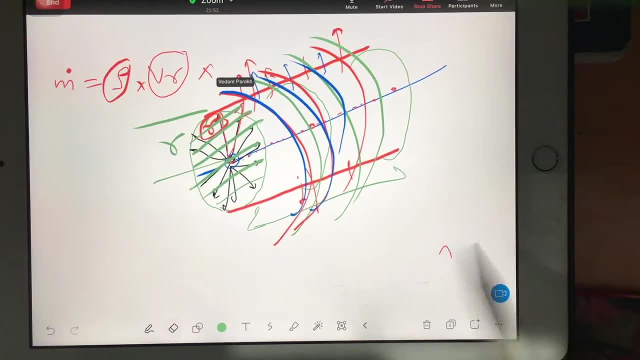 This is volume Pratik. what is your answer? Very good, 2 pi r h. 2 pi r h is the answer. Answer for the curvature: Curvature portion, Because from that portion only water is coming out. Okay, Water is not coming out like this. Try to understand my logic. So the area you 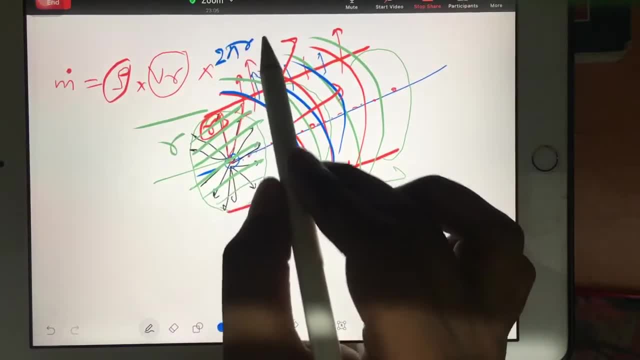 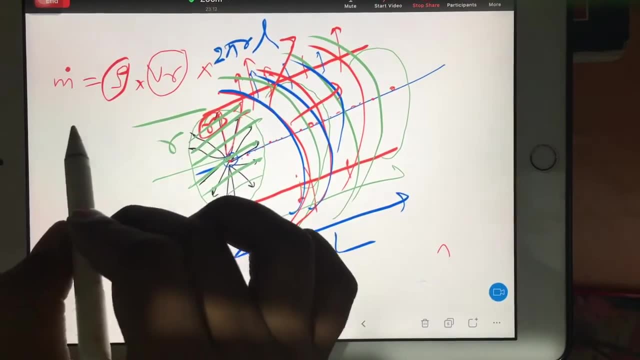 will replace as 2 pi r h, 2 pi r Now h. I am saying as a length, 2 pi r l, 2 pi r l. Okay, So see everything. whatever I have written here, it is not rocket science, Simply. 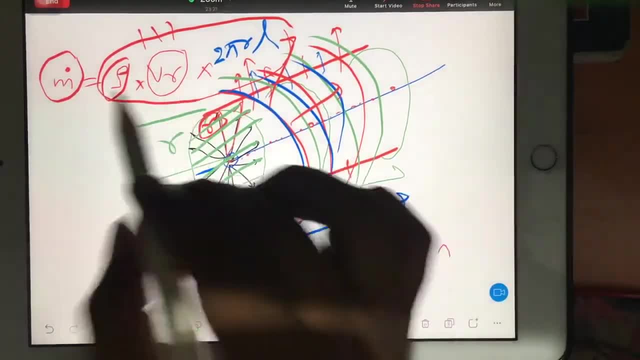 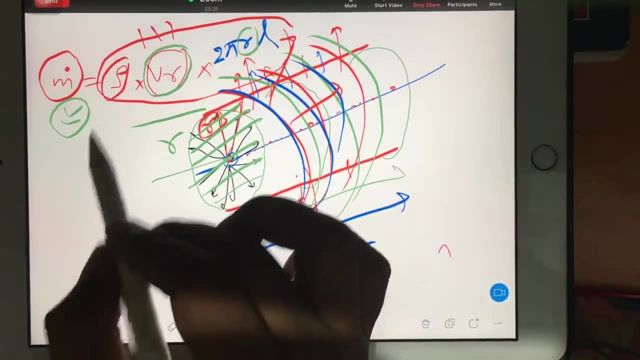 mass flow rate. anyone can find out. But try to understand. now, Here we got something very beautiful. We got v? r in the equation and r in the equation. It means we are on the right track to develop the equation in terms of v? r and r, v? r equation in terms of r. Now what is our next approach? Keep. 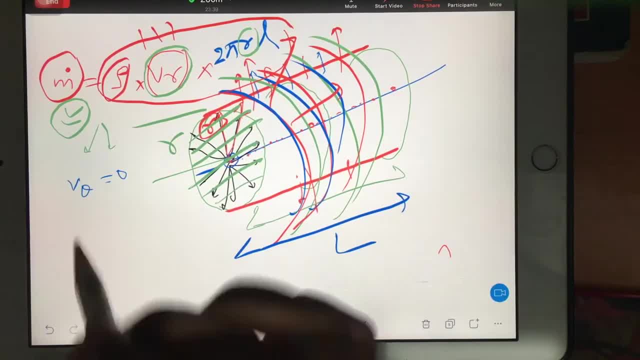 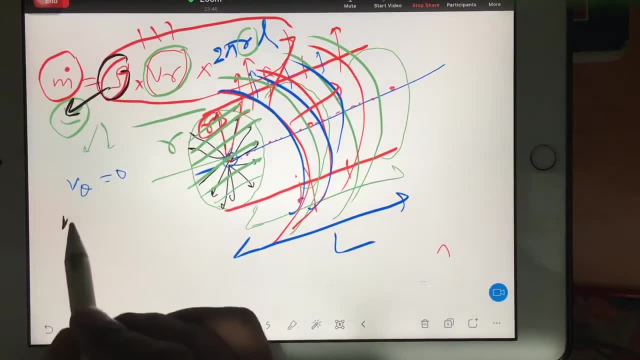 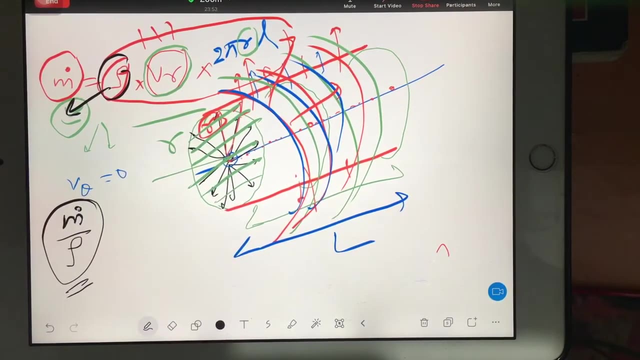 in mind: v? theta is 0.. Only v? r is finite. Okay, Tell me, if I will take this row, this side, then I will be getting this parameter. What will I call this? Tell me, Number 4.. No, not this. No, not this. No, not this sin theta. 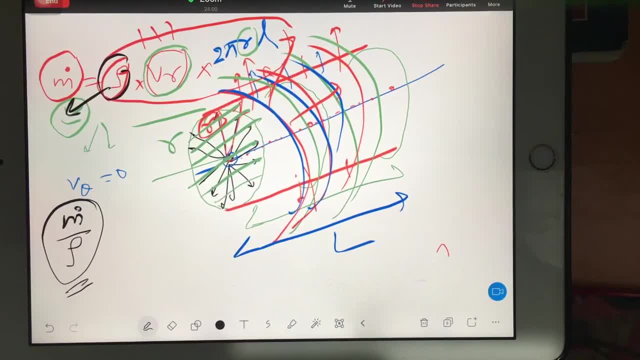 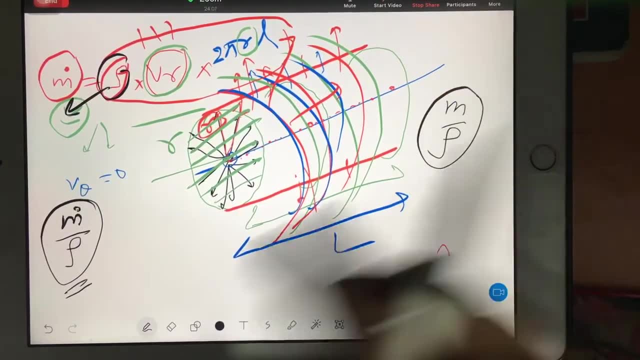 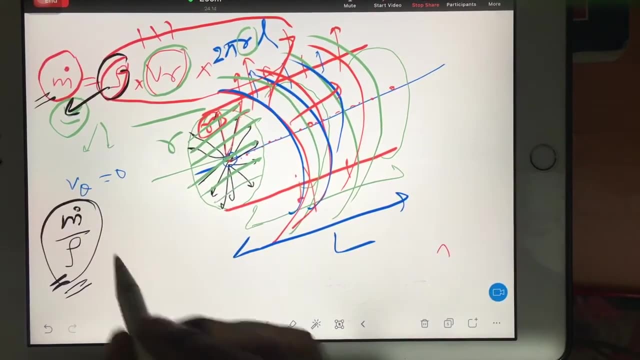 Sine theta 5000.. No, No, No, Everyone is capable to give this name Volume flow rate, Because mass by density is volume. So we started with mass flow rate equation. Now we got volume flow rate. Okay, So this is nothing but volume flow rate. So 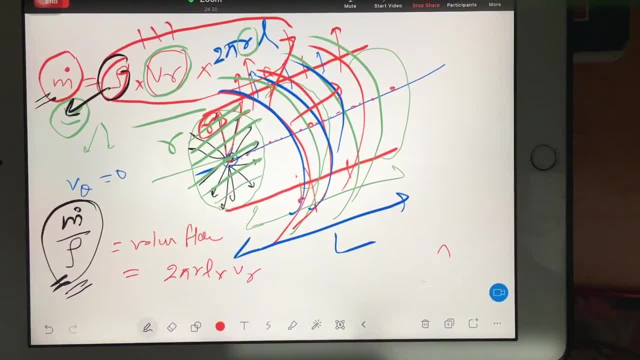 that is nothing but the remaining part. 2: pi R l into v? r. Okay, That is actually a number. again, I had written down the role, but actually I do not know the number of times since I will add it. Okay, The manually linear: proper finishing. 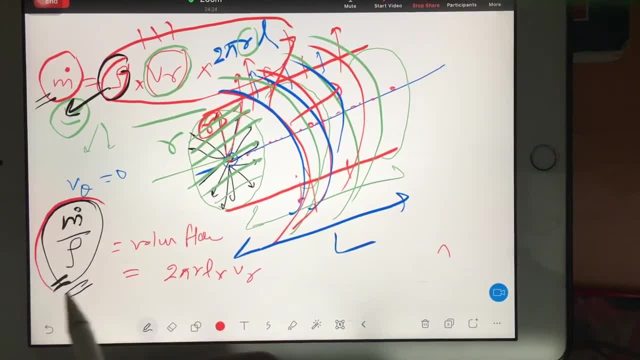 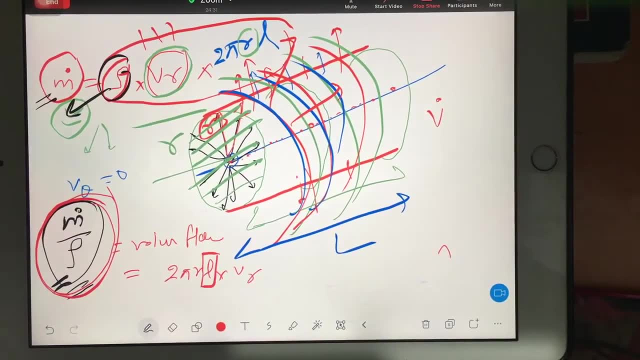 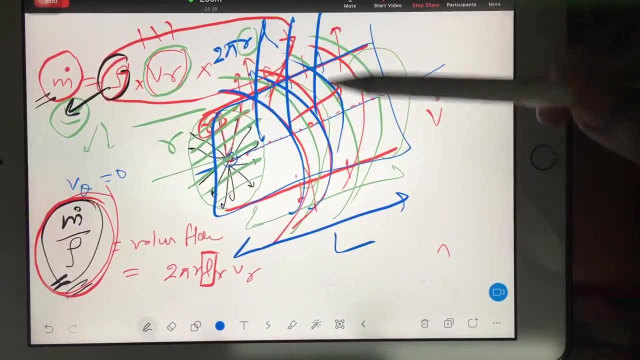 Anyway, I had как powerful pontos. Okay, Keep your function as straight as possible And at the now understand this total i can replace as v dot, so that v dot i will divide by this l. now you see, try to understand one logic. from this entire volume water is coming out. i will. 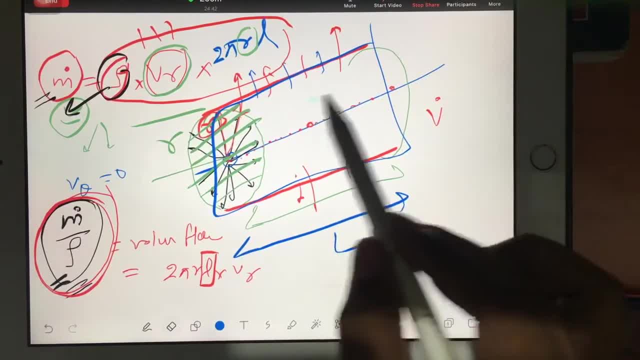 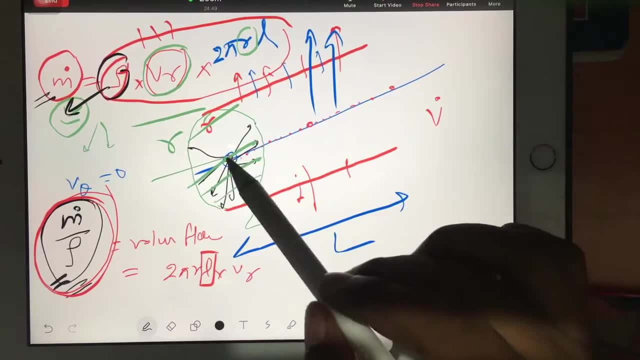 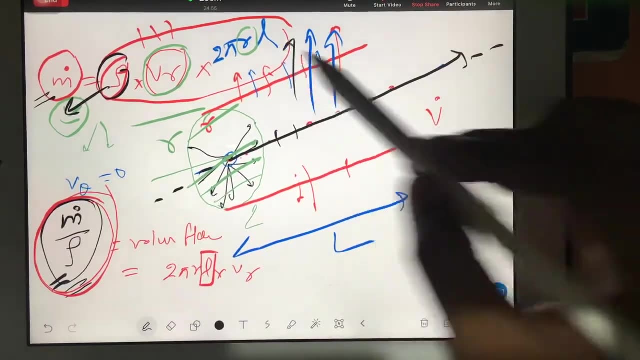 just erase this, for neat and clean purpose, from this entire volume. just a minute. water is coming out, water is coming out, so this length you can assume till any length, right till any uncertain length, because you have, because the water, the volume, what is coming out, that is because of 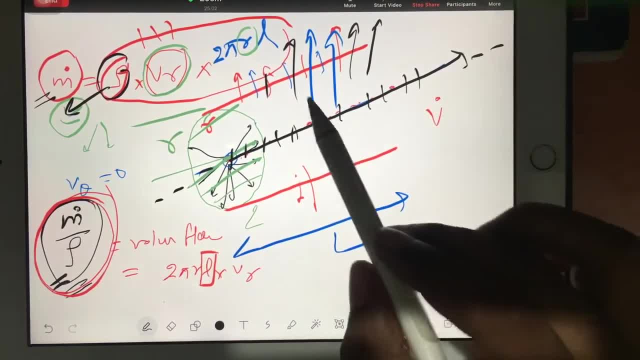 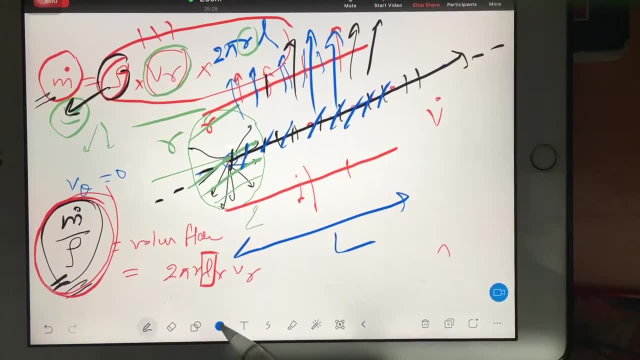 lot of sources. i am keeping on the way. i try to understand what i am saying. i am saying: this water, what is what is coming out? that is because of the all the sources, and where are the sources? they are sitting on the line. length of the line is l, but i am bothering about only one source. 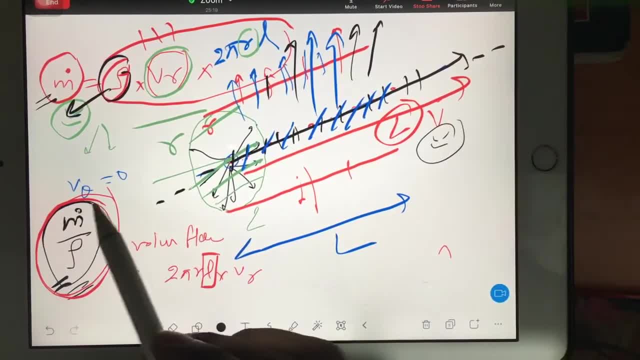 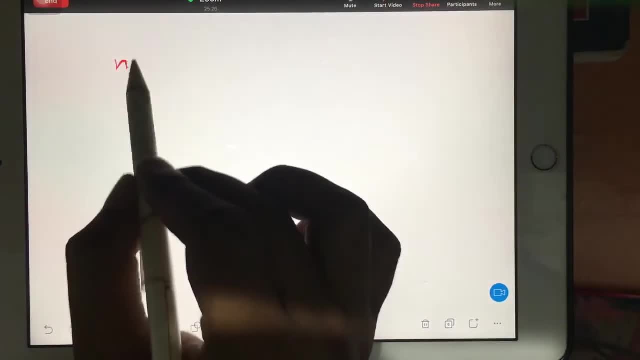 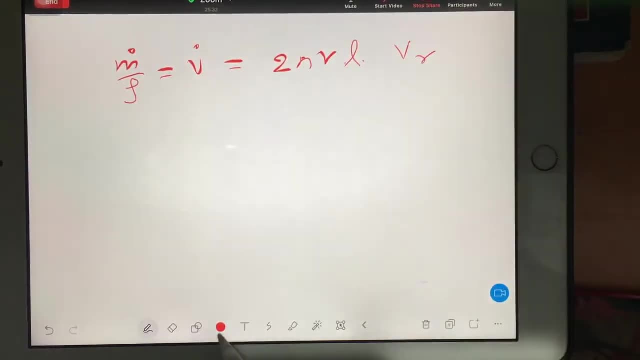 you, if you are bothering about the one source, then divide this entire equation by the l, then you will be getting unit length. it means your m dot by rho. you replace with v dot and write the entire equation: 2 pi r, then l, then v r and then you divide this entire volume flow rate. 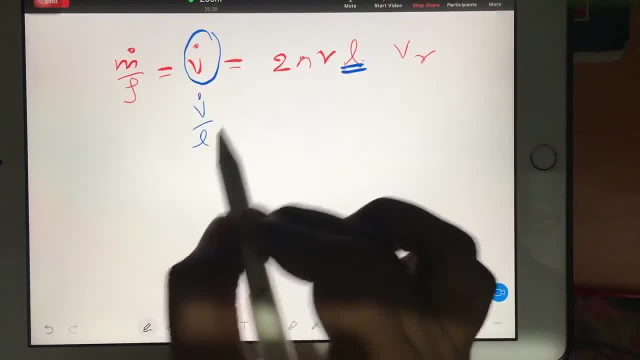 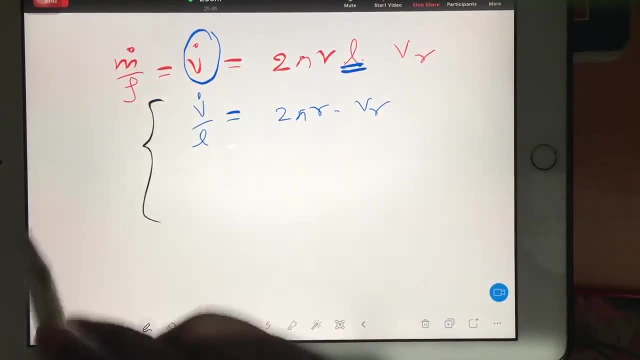 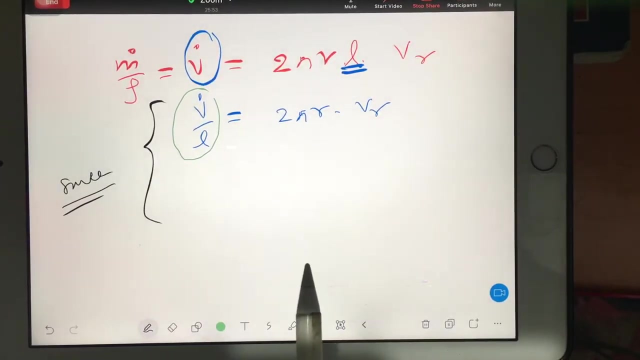 by the total length what you have assumed then it will be. v? dot by l is equal to 2 pi? r into v? r. see how easy this thing. from here only concept of source flow is started. this v? dot by l you will say as volume flow rate per unit length. 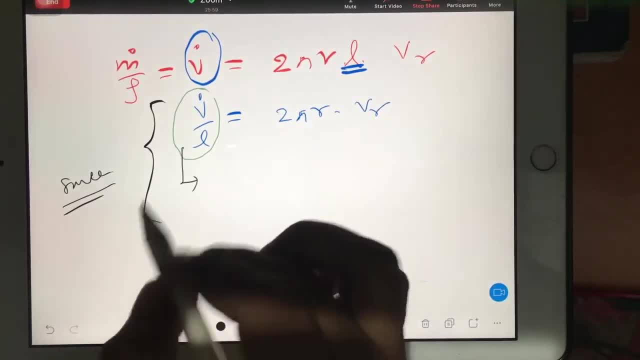 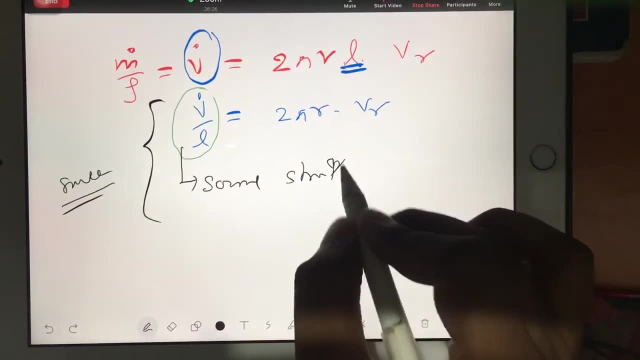 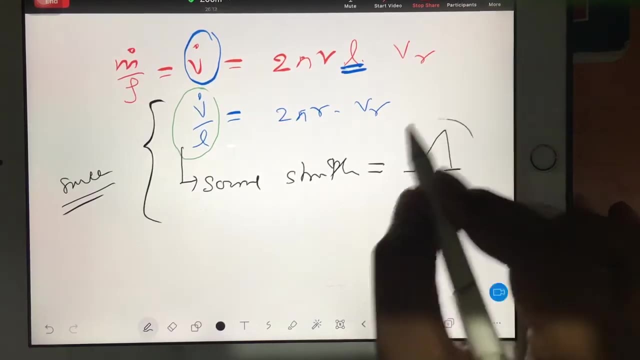 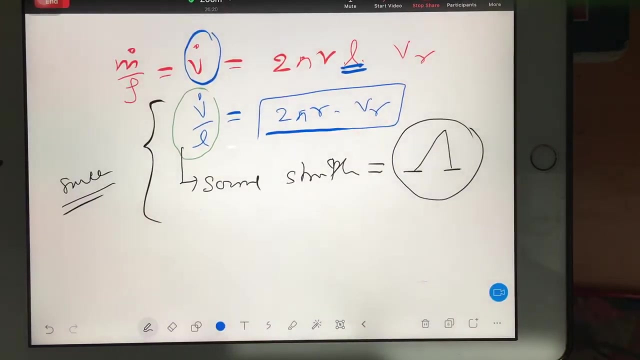 but it has a technical name. that technical name we say as source strength. you write the name properly: source strength. now this source strength, it has a symbol. that symbol is this: this is lambda: μ, μ, μ, ω? ν, γ, GM, λ, SC, capital. lambda is how much now this? 2 pi? r into v? r. so source is strength. we got now try to. 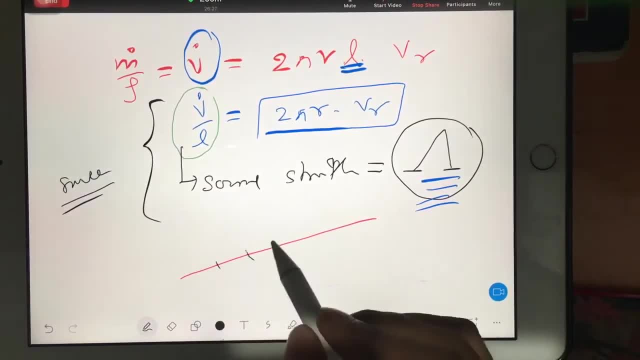 understand one logic on this length. i kept all types of all sources here, but maybe this source itself is of different, different capacity. this source can be very strong. this source can be very, very strong. this source can be extremely strong. so that's why we have to bother about source. 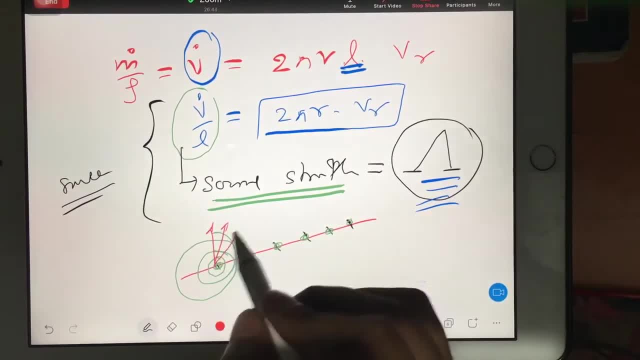 strength. it means what, how much velocity, or you can say how much mass flow rate this, this source, can develop. this is the physical meaning of source strength. okay, now understand, when you got the source strength, then you can replace, i mean you can rearrange the formulas. so that's all your v. 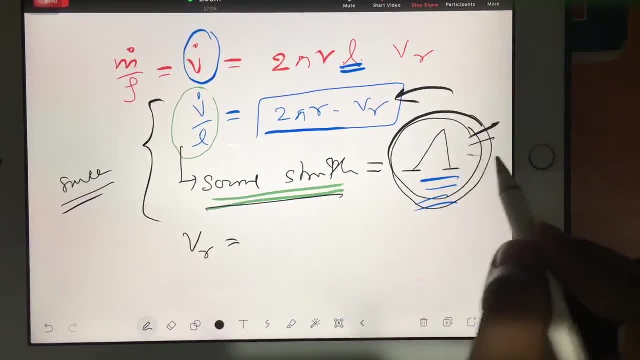 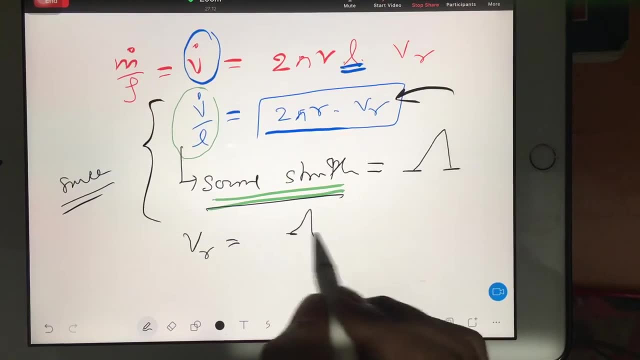 r. actually source strength is a personal quantity. personal quantity means it is a constant quantity for a given source, right? so this v? r is going to be source strength, capital lambda- keep in mind the name is capital lambda- divide by 2 pi? r. so right now we have developed our v? r equation in terms of r. so based on this equation, you can expect: 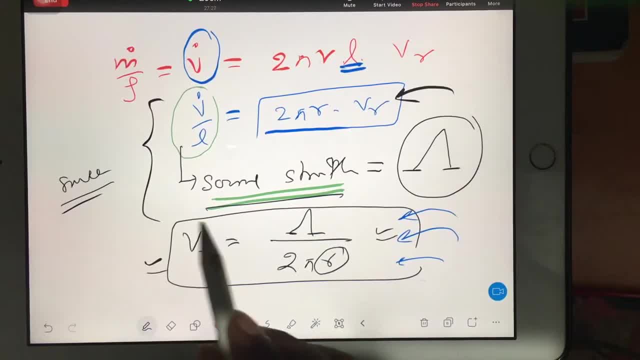 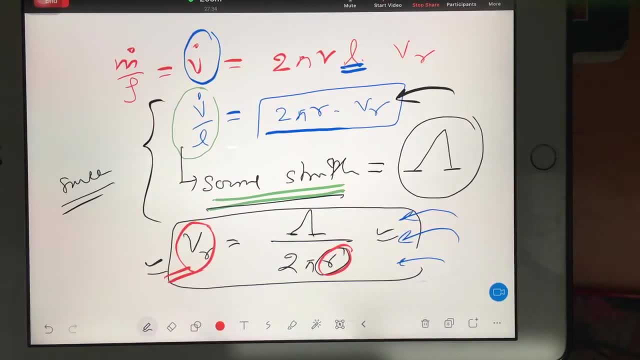 questions in gate exam. based on the relation between v? r and r, you can expect the question in gate exam. okay, now see this. v? r i will be using in the formula of psi and phi to develop the equation of psi and phi. i will change the page. 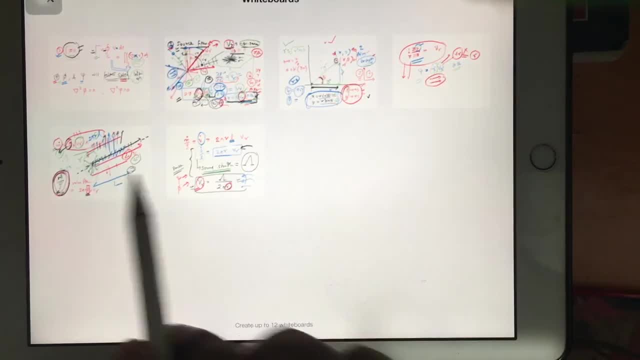 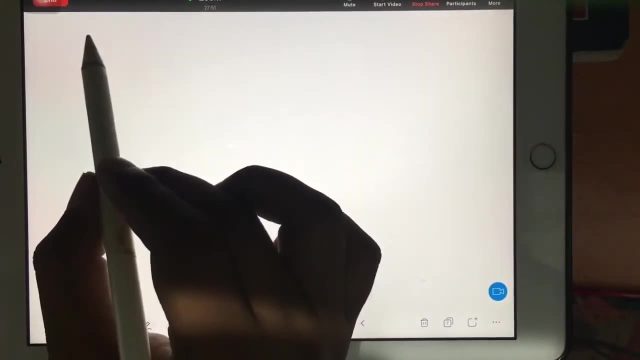 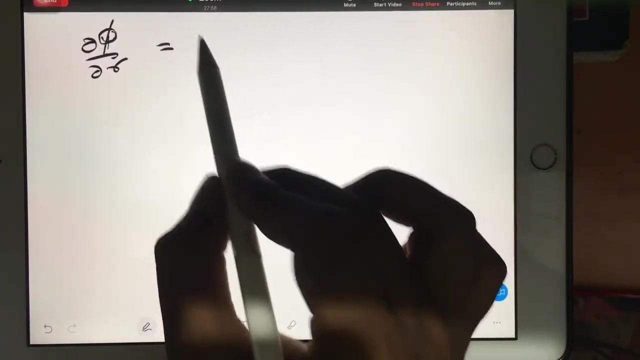 somewhere here we have formula. okay, i will. i will write the formula again. okay, so your dou phi by dou r, dou phi, i'm writing phi. dou phi by dou? r. formula was v? r, so just now we have got the equation of v? r. that v? r equation is nothing but your source. 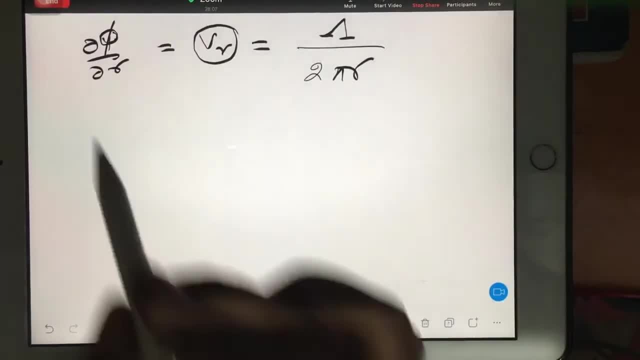 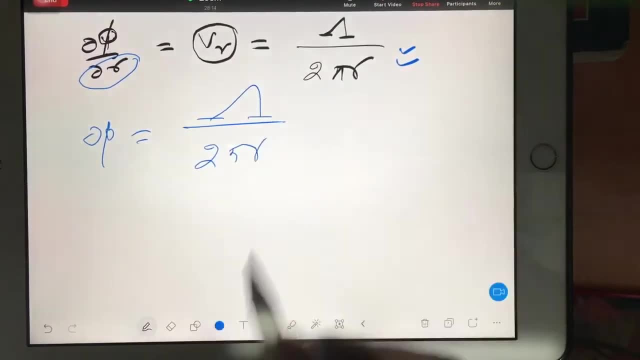 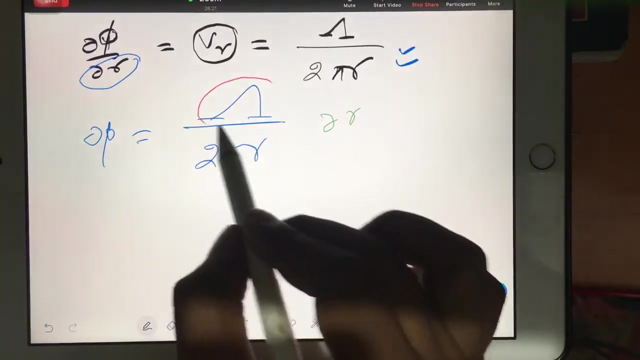 strength divide by 2 pi r. okay, now you take this r this side, so do phi will be your strength divide by 2 pi r. then here dou r now, no issues we can. we are free to integrate because this is constant value. this 2 is constant and this pi is constant. so when you 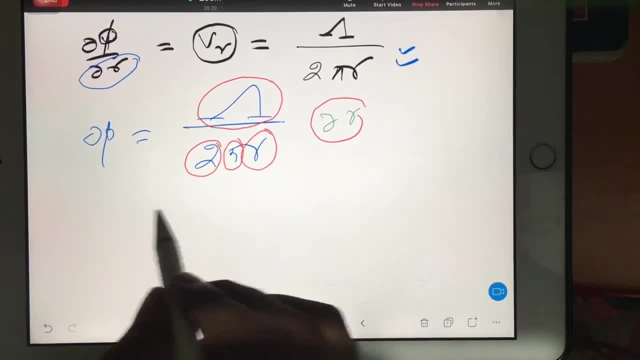 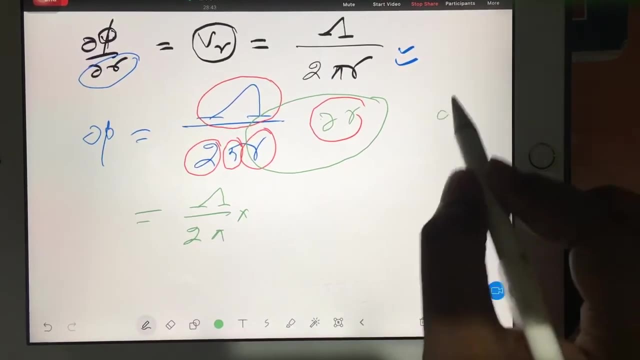 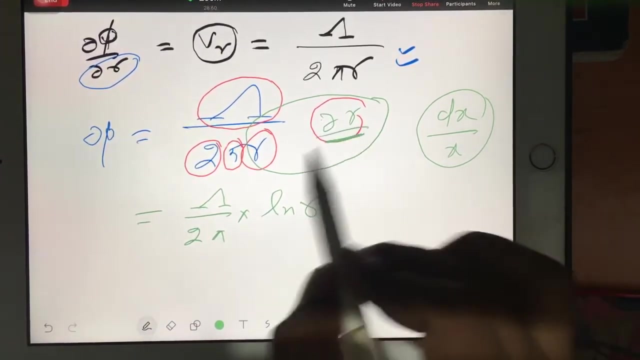 will differentiate this dou r and r quantity, sorry, integrate, so it is nothing. but tell me the answer. tell me the answer, you, Yes. So finally, whenever you keep in mind, whenever you differentiate dx by x, it gives natural log of x, sorry r. So here we are integrating dr by r, So it will be ln r.